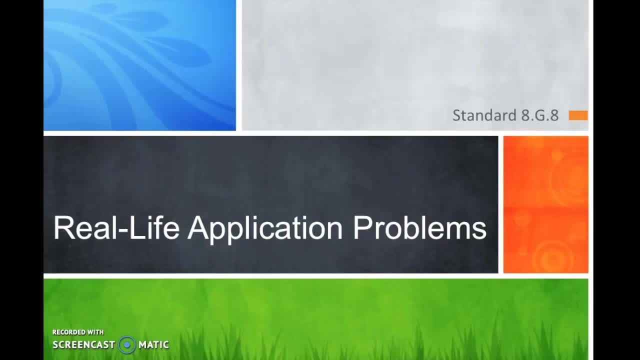 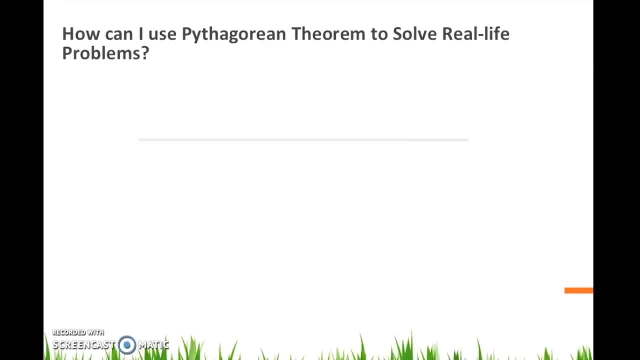 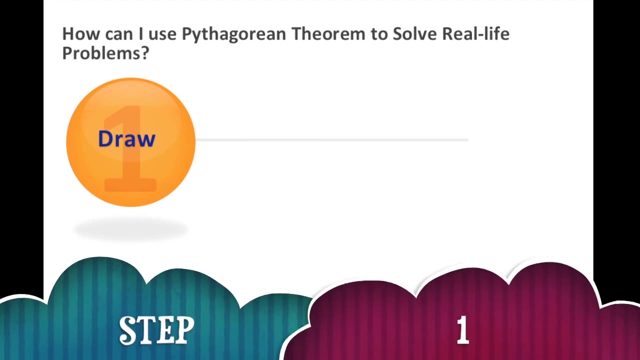 Today we're going to take a look at real-life application problems using Pythagorean Theorem. How can I use Pythagorean Theorem to solve real-life problems? We're going to use three easy steps. Step one: we're going to draw, we're going to use and we're going to solve. 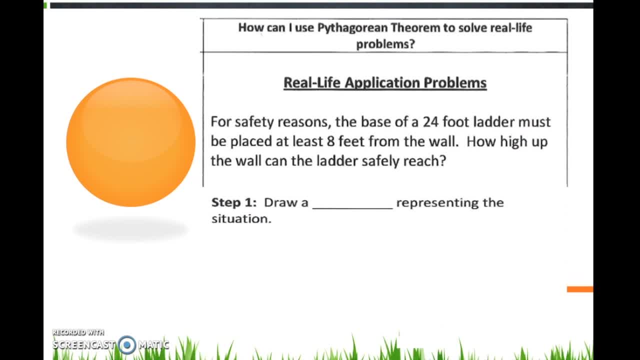 Let's read the real-life application problem. It says: For safety reasons, the base of a 24-foot ladder must be placed at least 8 feet from the wall. How high up the wall can the ladder safely reach? Step number one: draw a picture representing the situation. 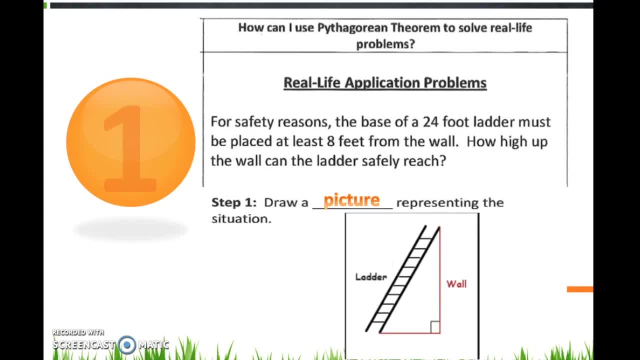 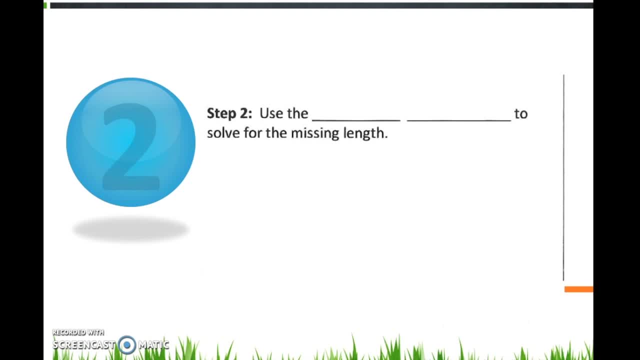 So here's our picture: a ladder placed at least 8 feet from the wall. Step two: we're going to use the Pythagorean Theorem to solve for the missing length. a squared plus b squared equals c squared. They gave us c, they gave us b. 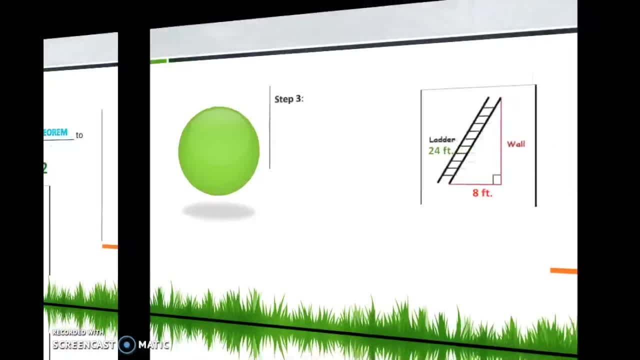 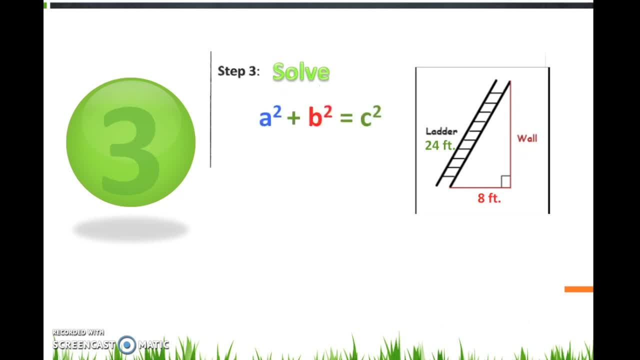 a is what's in question. Step three we're going to solve Using the information given. we're going to plug it into our formula: a squared plus b squared equals c squared. So we have a squared plus 8 squared equals 12.. 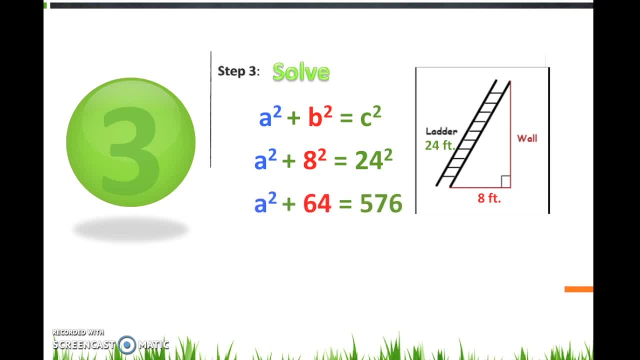 24 squared 8 squared 64.. 24 squared 576.. We're going to do the inverse operation. Subtract 64 on both sides, leaving us with a squared is equal to 512.. How do we undo a square? 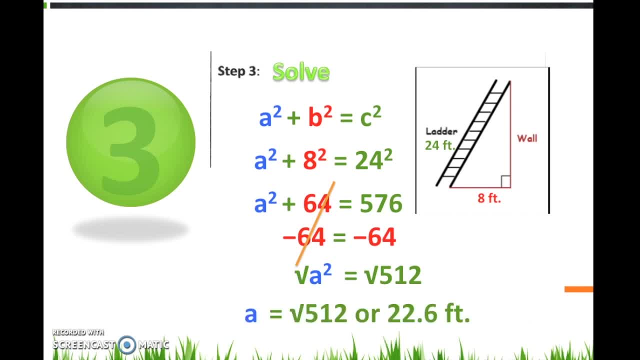 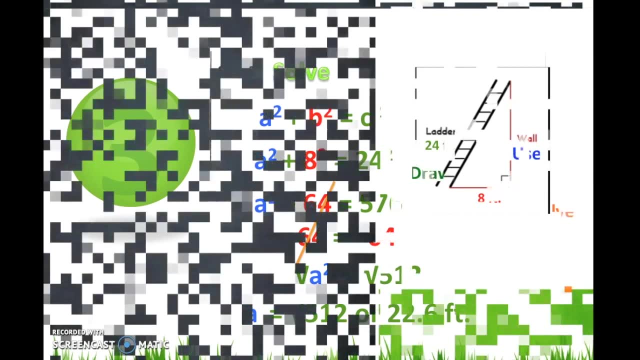 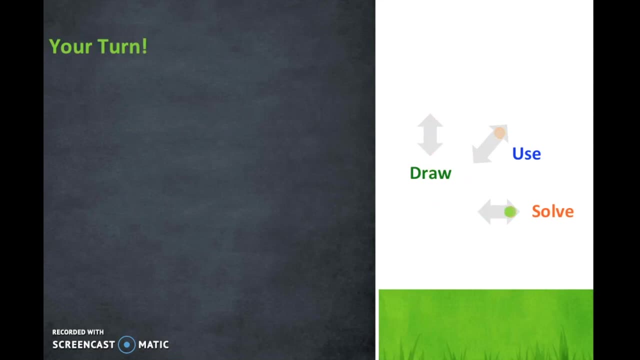 We find the square root a is equal to the square root of 512, or 22.6 feet. Hope that's making sense. Now it's your turn, So you're going to draw, use and solve the given problem. 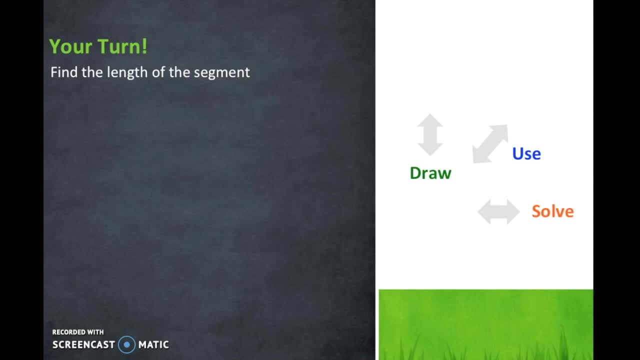 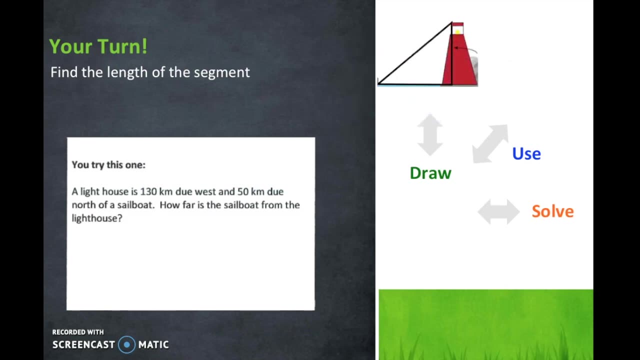 First you're going to do is find the length of the segment. So pause the video and give it a try. Let's see what you got. So, step one: you're going to draw that picture, So I'm going to give you a chart that's going to help you extract the key words.